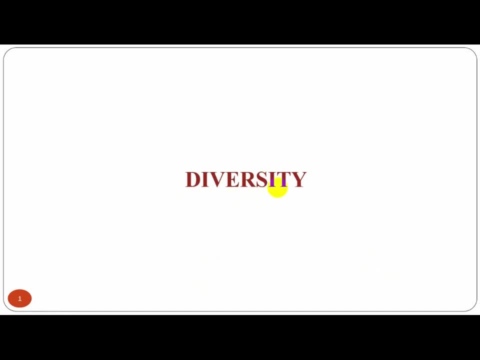 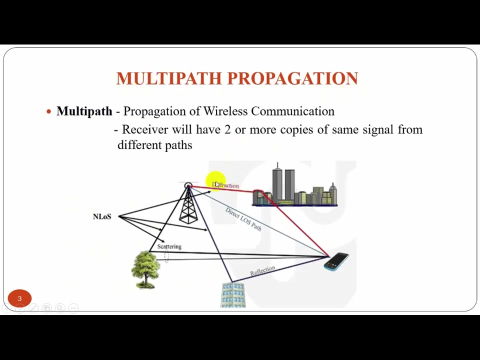 In this video we are going to discuss about the topic diversity. The contents of this presentation includes principles of diversity, need for diversity, types of diversity, types of micro diversity and diversity combining techniques. We have already learned about multipath propagation In wireless communication. 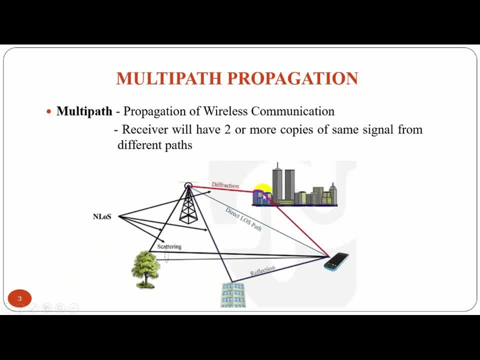 the information is transmitted in multiple paths. Either it can be a direct line of sight path, otherwise, because of diffraction, reflection scattering, it can take multiple paths to reach to the destination. So the receiver will get two or more copies of the same signal from different paths. The principle of 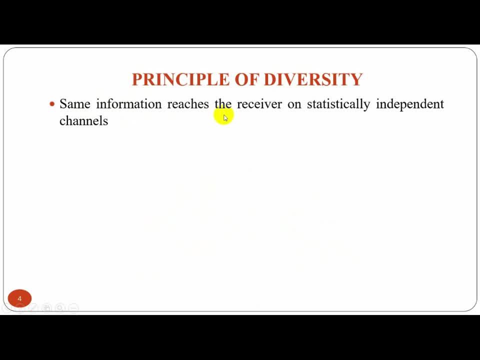 diversity is to ensure that the same information reaches the receiver on statistically independent channels In multipath propagation. if one radio path undergoes a deep fading, another independent path may have strong signal. So the receiver can choose the strong signal By having more than one path to select from, both the instantaneous and 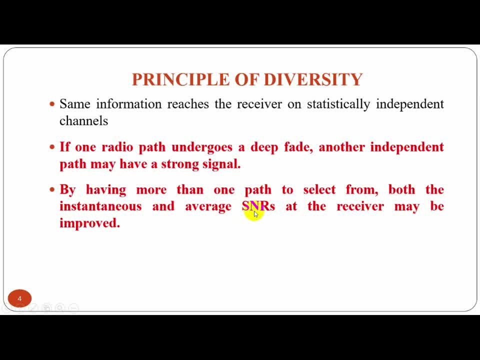 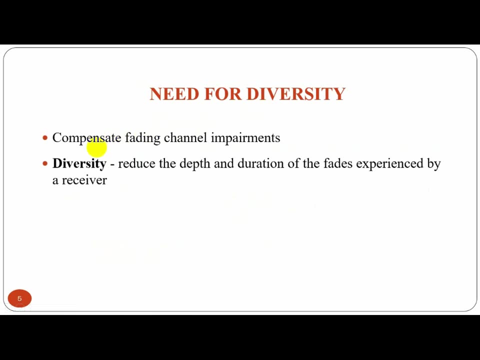 average signal to noise ratio at the receiver may be improved. Diversity can be provided across time, frequency and space. The need for diversity In wireless communication. the fading effects of the channels are unavoidable. We have to compensate the fading channel impairments. Diversity actually reduces the depth and duration of the fades. 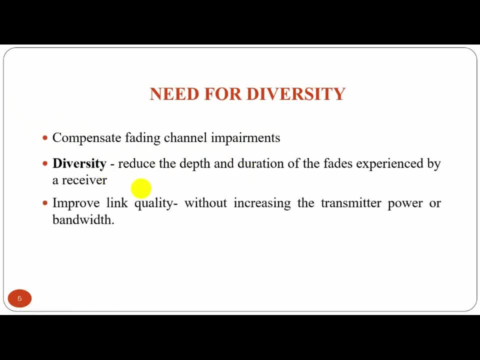 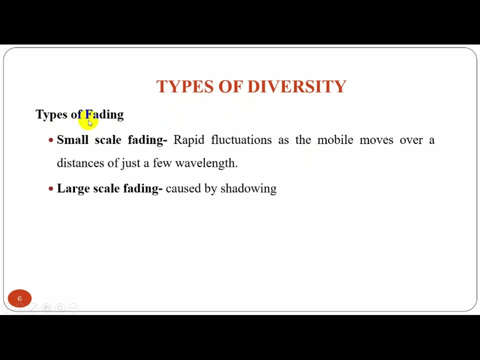 experienced by the receiver. Diversity also improve the link quality without increasing the transmitted power and bandwidth. Now we are going to see the types of diversity. We know the types of fading, that is, small-scale fading and large-scale fading. Small-scale fading creates rapid fluctuations when the user is moving through a small distance of. 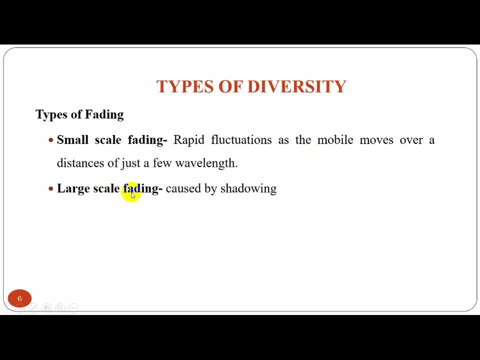 just few wavelength. Large-scale fading is caused by shadowing. Diversity is basically divided into microdiversity and macrodiversity. Microdiversity: it is used to reduce small-scale fading effects of the channel. Macrodiversity is: 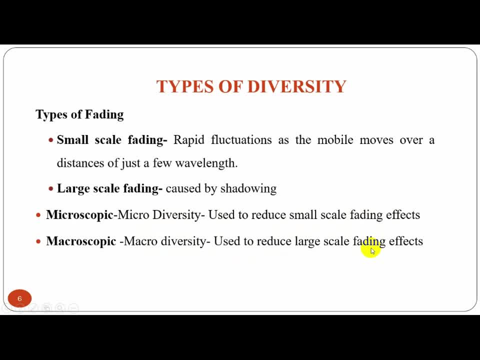 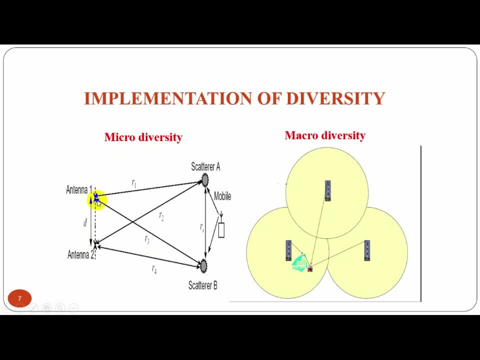 used to reduce large-scale fading effects of the channel. In microdiversity, two antennas are separated by a small distance. One, Andreanum, may receive a good signal. other, antonite, may receive a faded signal In macrodiversity. 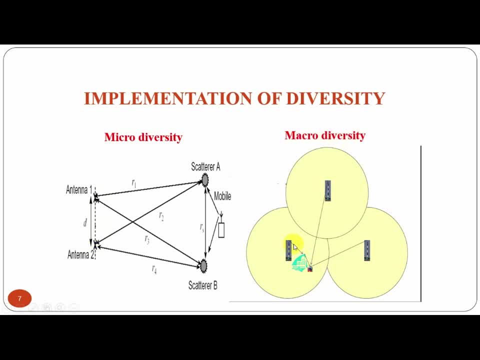 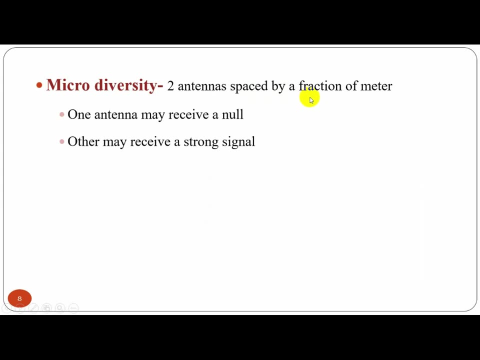 the receiver has to choose the base station which is not shadowed. Here this base station is shadowed, so the receiver has to choose any other base station. So in microdiversity, two antennas are spaced by a fraction of meter. that is a small. 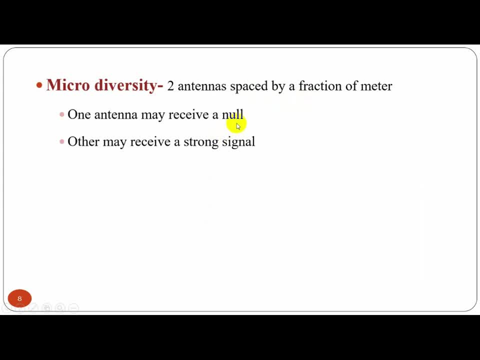 distance. One antonym may receive no signal. other antonym may receive a strong signal, So the receiver can choose the strong signal. For macro diversity, the receiver has to select a base station which is not shadowed when others are in the shadowed region. 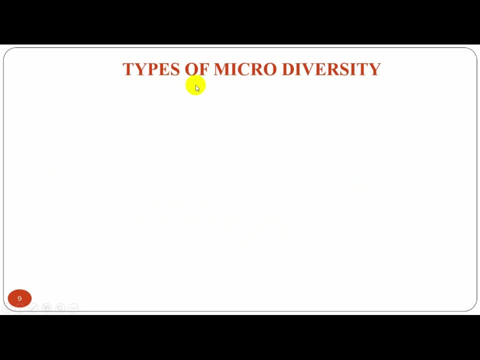 In this we are going to see the types of micro diversity. Diversity describes different ways of obtaining the statistically independent copies. We concentrate on the methods that can be used to combat small scale fading, which are therefore called as micro diversity. Here we are going to see about the receiver diversity. 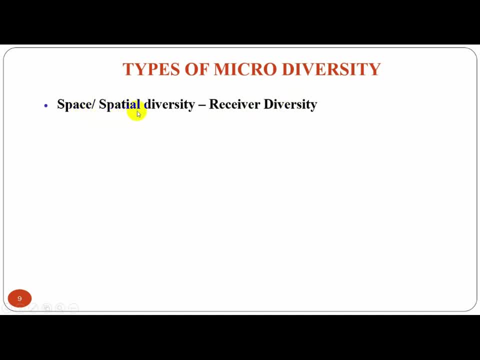 The first type of micro diversity is space or spatial diversity. Here several antenna elements are separated in space. These are the types of spatial diversity That is, selection diversity, Feedback diversity, Maximal ratio combining And equal gain combining. This maximal ratio combining and equal gain combining are the diversity combining techniques. 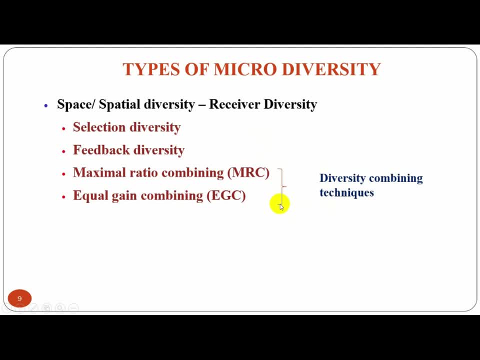 We are going to detail study this in this video. Next is the time diversity or temporal diversity. Here, the signal is transmitted at different times. Next is the frequency diversity. Here, the signal is transmitted at different times. This means that the signal is transmitted at different frequencies. 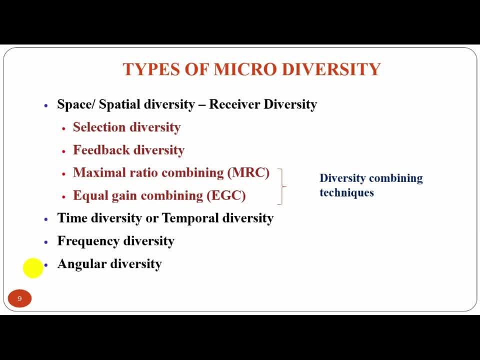 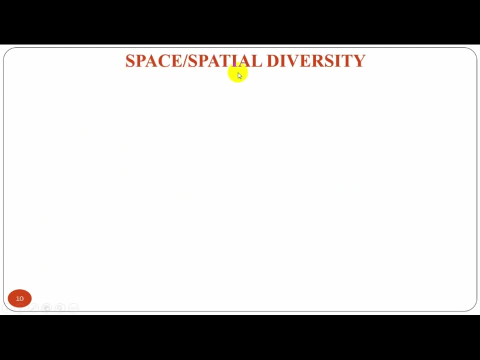 Next is the angular diversity. Here we are going to use multiple antennas with different antenna patterns. Next is the polarization diversity. Here multiple antennas with different polarizations are used. That is, vertical polarization, horizontal polarization. Now we are going to see about space or spatial diversity. 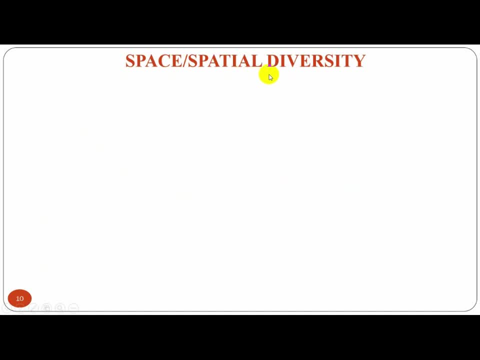 The third type of micro diversity. This is the spatial diversity and simplest form of diversity and it is most widely used. It is the antenna diversity. Here multiple antennas are used. The antennas are separated on the order of several turns of wavelength and the signals must have high D. 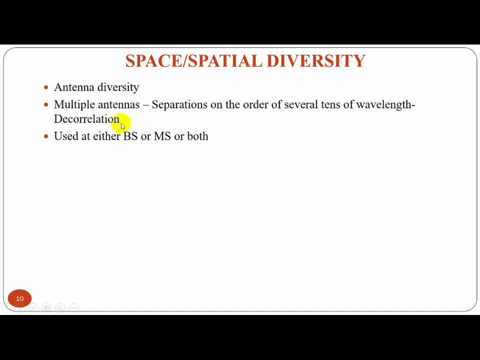 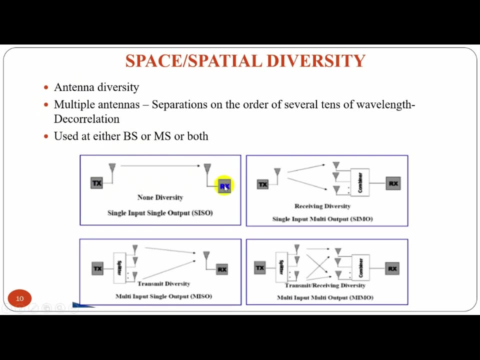 correlation. If the signals are highly correlated, there is no use of diversity technique. Diversity can be used at either base station or mobile station, or both at base station and mobile station. If you are using single transmitter and receiver, there is no diversity technique. Here, at the receiver side, we are having 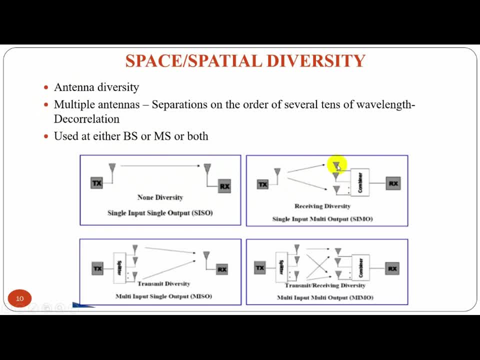 multiple antennas. so it is a receiving diversity technique. So here we are having single input and multiple output SIMO systems. Here at the center side we are having multiple antennas. so this is a transmit diversity technique. This is multiple input and multiple output. single output MISV system. in this diagram we can see at the transmitter. 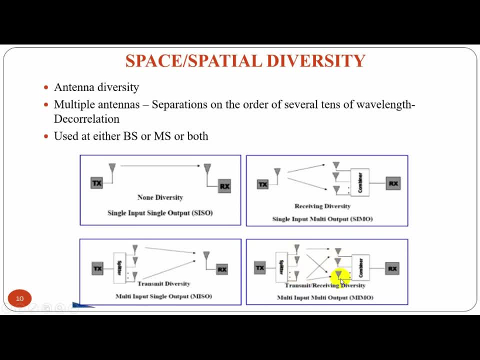 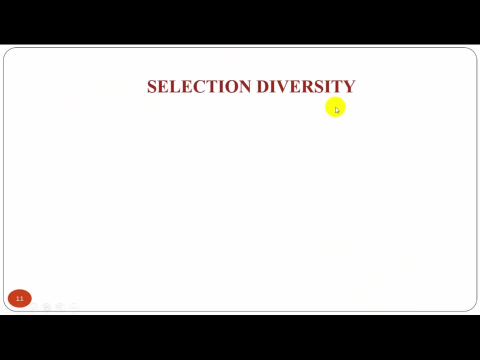 side also diversity technique is used. at the receiver side also diversity technique is used. so here we are having multiple input, multiple output. that is MIMO system, otherwise MIMO systems. now we are going to see the types of spatial diversity. first one is the selection diversity. this is a simple 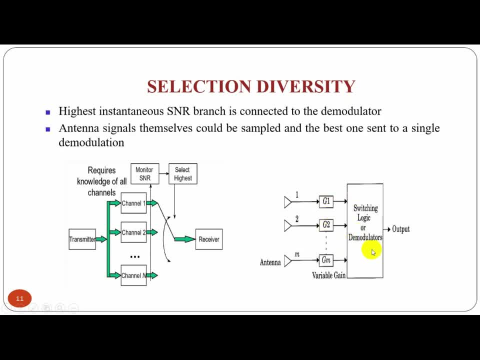 diversity technique. here M demodulators are used to provide M diversity branches whose gains are adjusted to provide the same average signal to noise ratio for each branch. the receiver branch which has the highest instantaneous SNR is connected to the demodulator antenna. signals themselves could be sampled and the best one is sent to the. 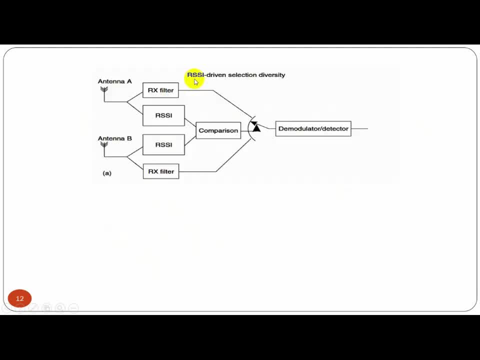 receiver single demodulator. this is one example for RSSI driven selection diversity. that is received signal strength indicator. so the received signals from different ANNAS, the signal strength, is measured and which one is having the highest signal strength. that is connected to the demodulator is an. 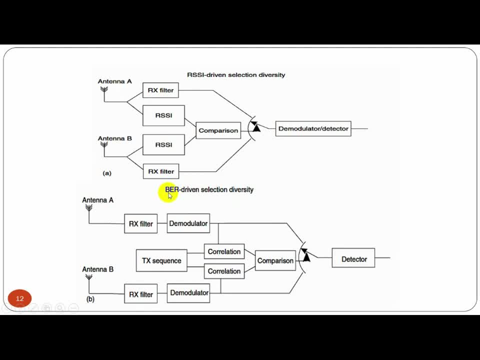 example for BER driven selection diversity, that is, bit error rate driven selection diversity. here the received signal is demodulator and is correlated with the transmitter sequence, which is having high correlation, which is connected with the detector, so the error will be less facial diversities, feedback or scanning. 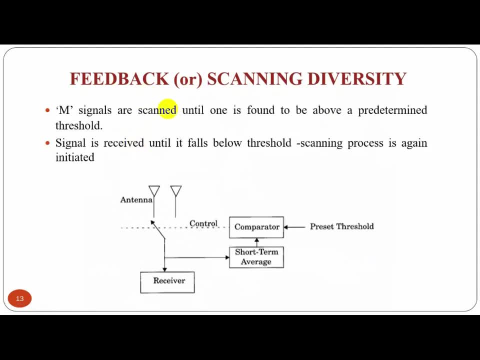 diversity. scanning diversity is very similar to the selection diversity, except that instead of always choosing the best of M signals, M is the best of M channels. Then signals are scanned until one is found to be above the predetermined threshold. This signal is then received until it falls below the threshold. 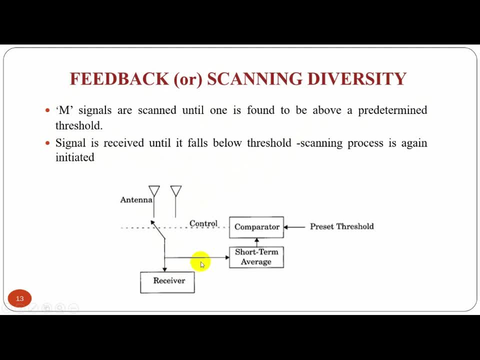 Then the scanning process is again initiated. The resulting fading statistics are somewhat inferior to that obtained by other methods. The advantage of using this method is it is very simple to implement. Only one receiver is required. Next type of spatial diversity is maximal ratio combining. 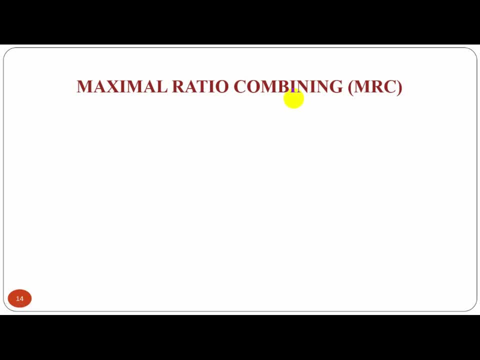 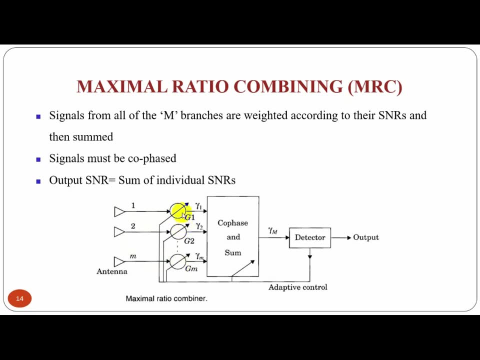 This is coming under diversity combining technique. Here the signals from all the M branches are weighted according to their individual signal to noise power ratios and they are added up. Here the individual signals must be co-phased before it is summed. It generally requires an individual receiver and phasing circuit for each antenna element. 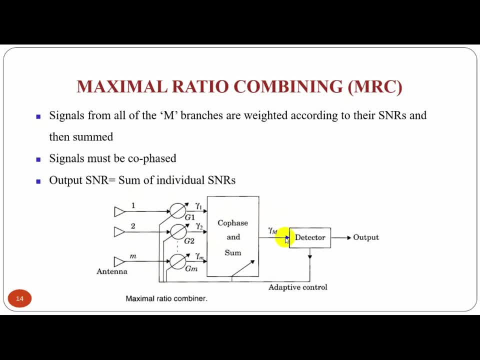 Maximal ratio. combining circuit produces an output SNR equal to the sum of individual SNRs. The advantage of using this technique is it produces an output with an access to the signal. This is acceptable SNR, even when none of the individual signals are themselves acceptable. 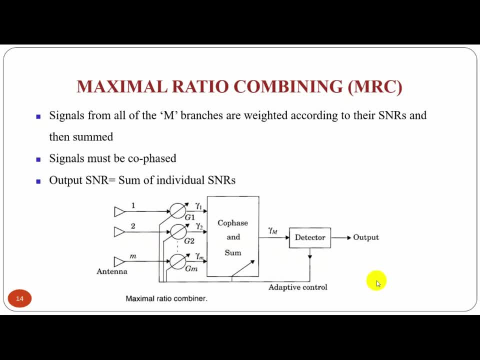 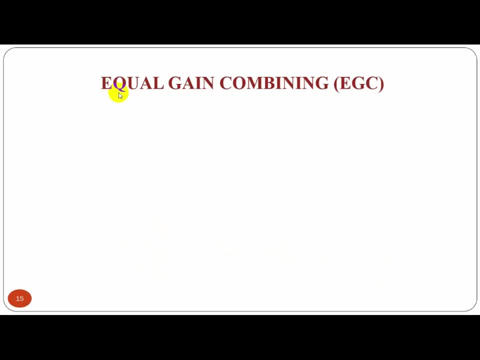 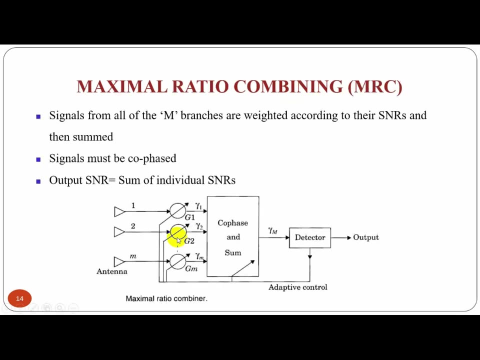 This technique gives best statistical reduction of fading of any known linear diversity combiner. Next, spatial diversity technique is equal gain combining technique, which is also a diversity combining technique. In certain cases it is not convenient to provide the variable weighting capability required for the maximal ratio combining. 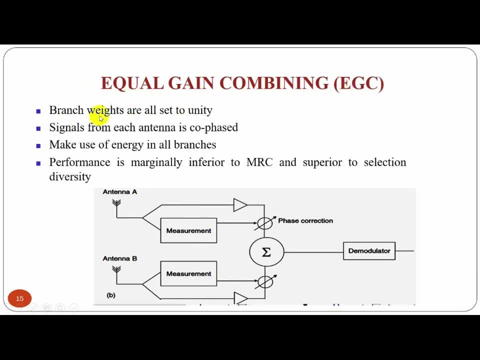 So in equal gain combining technique, the branch weights are set to unity, but the signals from each branches are co-phased to provide equal gain combining diversity. This allows the receiver to exploit the signals that are simultaneously received on each branch. The possibility of combining is very high. 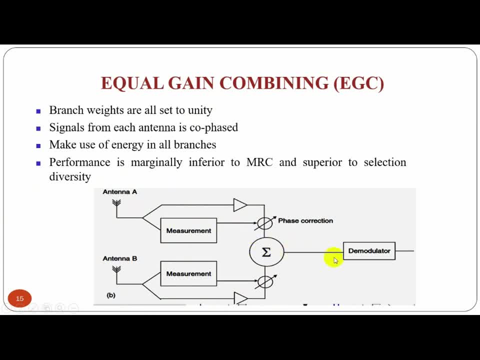 So in this case it is not convenient to provide the variable weighting capability required for the maximal ratio combining. The probability of producing acceptable signal from a number of unacceptable input is still retained. The performance is only marginally inferior to maximal ratio combining, but superior to. 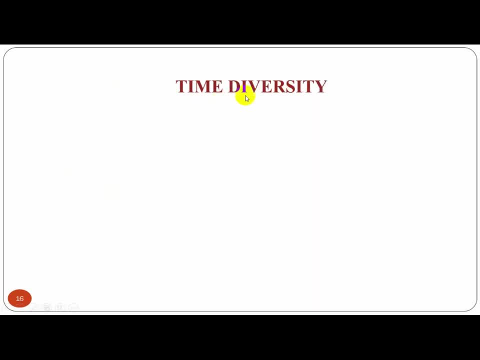 selection diversity. The next type of microdiversity is time diversity. The wireless propagation channel is time variant, so the signals that are received at different times are uncorrelated. So the signal that is received at different times are uncorrelated. Here the transmitter repeatedly transmits the information at different times. 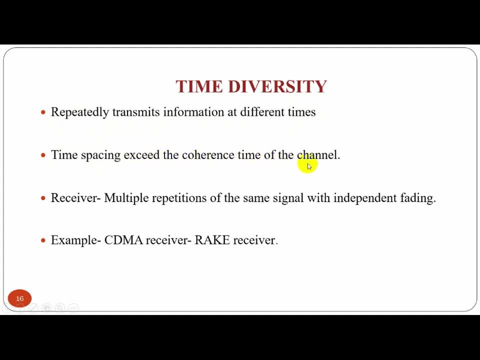 The time spacing must exceed the coherence time of the channel. then only the signals are de-correlated. At the receiver side, multiple repetitions of the same signal we will receive, with independent fading. This time diversity is implemented in the rack. receiver Time diversity or terminal diversity is realized by the signal that is transmitted to the 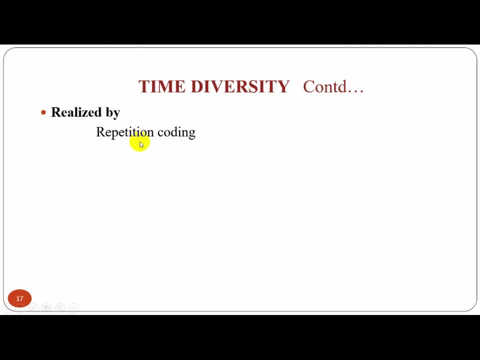 receiver by different ways. The first one is repetition coding. Here the signal is repeated several times, where the repetition intervals are large enough to achieve de-correlation. But the disadvantage is it is highly bandwidth inefficient. The spectral efficiency reduces by a factor that is equal to the number of repetitions. Next technique is automatic repeat request. 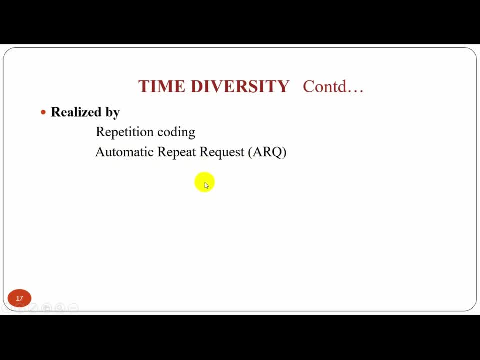 Here the receiver sends messages through the transmitter to indicate whether it received the data with sufficient quality. If not, the transmission is repeated. Spectral efficiency of ARQ is better than the repetition coding. In ARQ, multiple transmissions recurs only when the first transmission occurs in a bad, fading state. ARQ recurs a feedback channel. 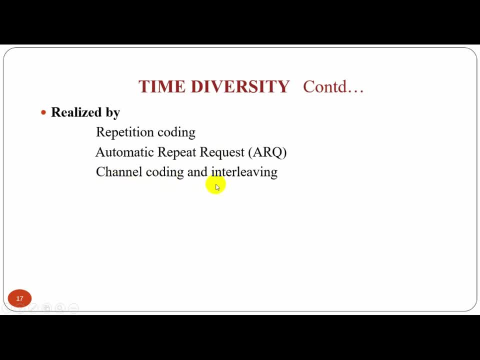 Next technique is channel coding and interleaving. The more advanced version of repetition coding is forward error correction coding. with interleaving, Different symbols of code words are transmitted at different times, which increase the probability that at least some of them arrive with a good signal to noise ratio. 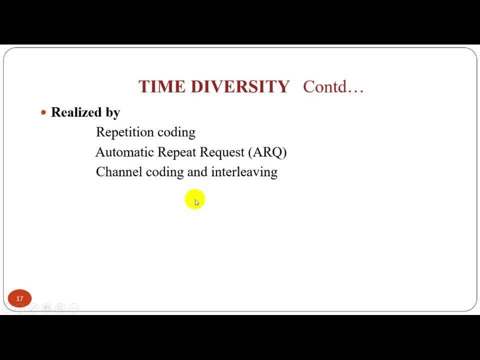 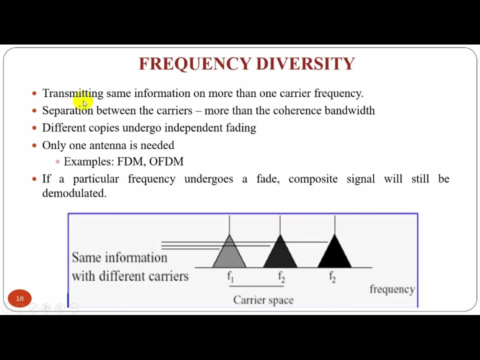 The transmitted code word can then be reconstructed. The disadvantage of this method is it wastes the bandwidth and affects the delay. Next micro diversity technique is frequency diversity. Here the same signal is transmitted at two or more different frequencies. If the frequencies are separated apart, then the coherence bandwidth of the channel fading. 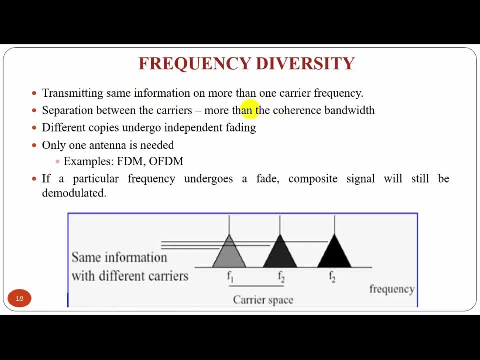 is approximately independent, And the probability is low that the signal isn't de-fade at both frequencies simultaneously. Here different copies undergo independent fading In frequency diversity. we require only one antenna. Examples for that will be frequency division, multiplexing, orthogonal frequency division. 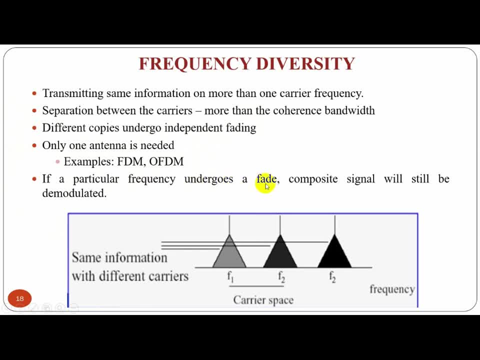 multiplexing. If a particular frequency undergoes a fade, a composite signal will still be demodulated. The difficulty of this frequency diversity is it is not common to actually repeat the same information at two different frequencies. This greatly degrees spectral efficiency. 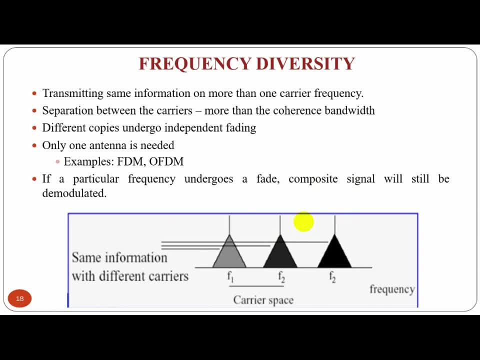 So the solution for that is, the information is spread over the large bandwidth so that small parts of the information are conveyed by different frequencies to recover the original information. This spreading can be done by different methods like CDMA, multi-carrier CDMA, and so on. 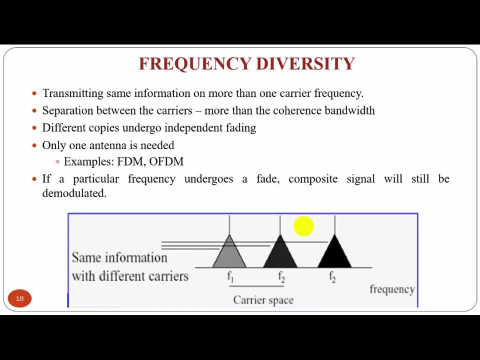 In this way, the information is spread over the large bandwidth, so that small parts of the information are conveyed by different frequencies to recover the original information. This way, the information is spread over the large bandwidth, so that the information is spread over the large bandwidth, so that the information is spread over the large bandwidth. 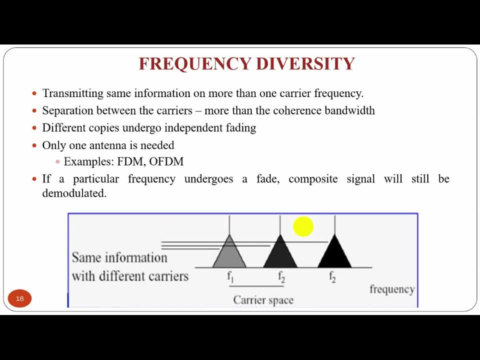 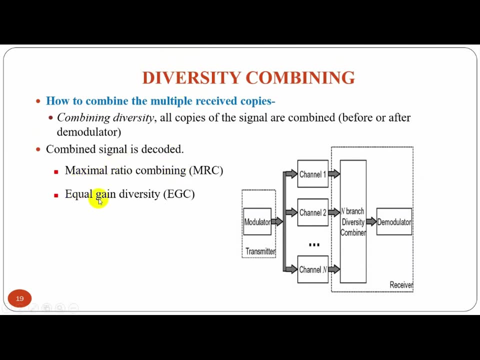 Frequency hopping in conjunction with coding, These methods allow the transmission of information without wasting the bandwidth. These are the diversity combining techniques which we already discussed. That is, maximal ratio combining and equal gain diversity Combining diversity. all copies of the signals are combined, before or after demodulator. 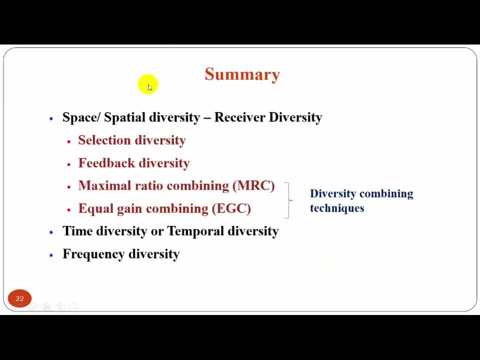 You can see that the signal is much smaller than the original signal. so in this video we have discussed about types of microdiversity. the first one is space or spatial diversity, and the types of spatial diversity: selection diversity, feedback diversity, MRC, EGC. then we have learned about time diversity, or temporal. 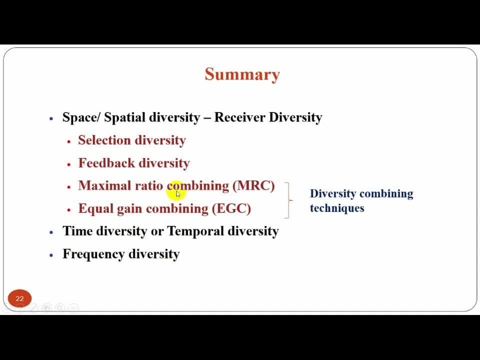 diversity and frequency diversity. this maximum ratio combining and equal gain. combining are the diversity combining techniques. thank you for watching this video. 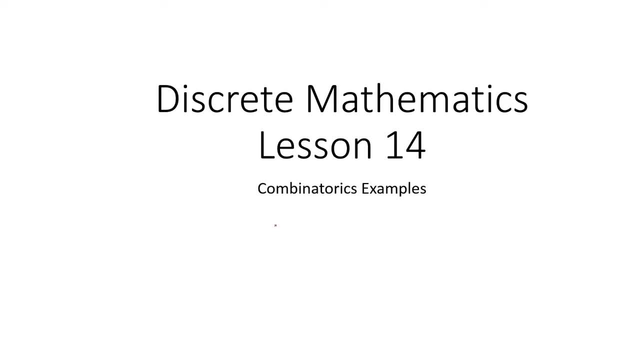 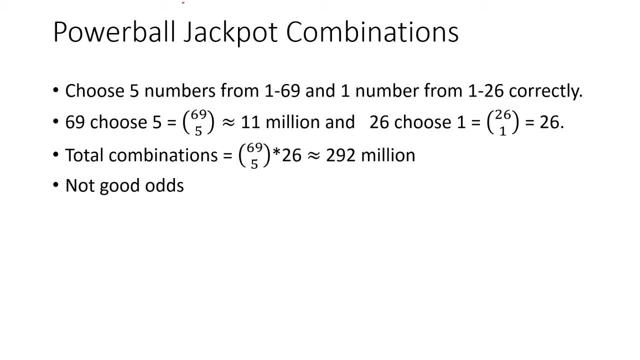 Hello and welcome back to ScreetMath. This is lesson 14.. We're going to be going over some combinatorics examples, So the first one we're going to do is computing the number of ways, the number of possible Powerball tickets. So the way the Powerball works is. 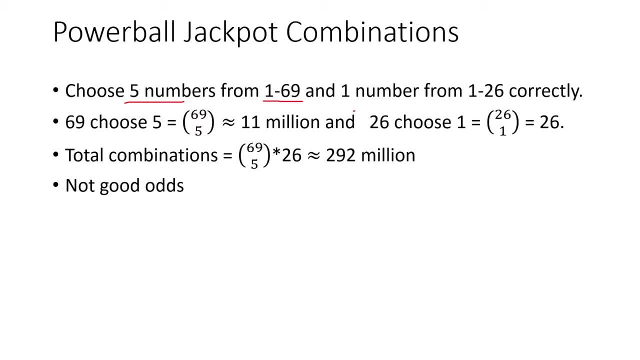 you choose five numbers from 1 through 69, and then we choose one number from 1 to 26, and if we get all those correct, we win a big jackpot. So we're going to compute the number of ways that could happen. So we first compute 69, choose 5, and that is around 11 million. 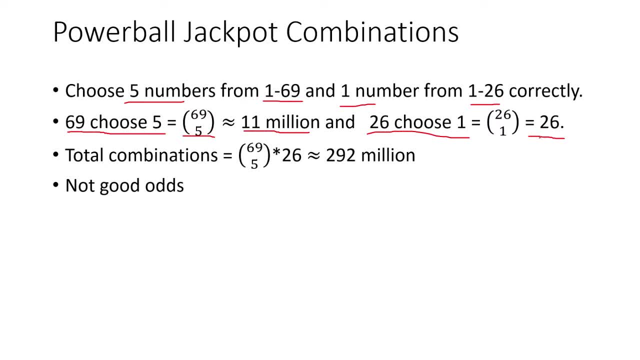 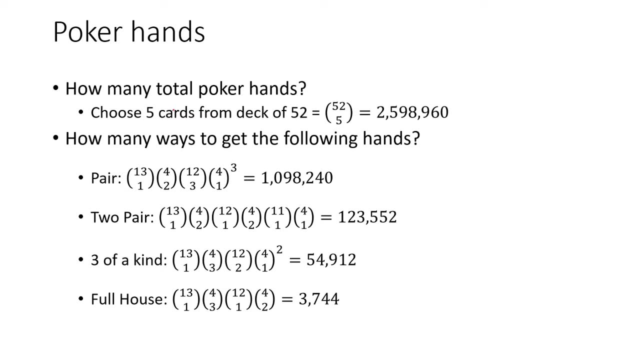 and then we compute 21, choose 6, which is just 26, and then we can all apply those two numbers together and we'll get around 229 million possible tickets. So not very good odds for you to get one of those. Next will be poker hands. We're going to compute a number of 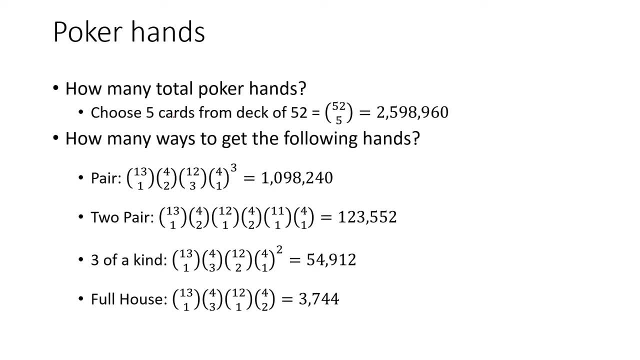 different poker hands. So first we're going to compute the total number of poker hands, and the way poker works is you choose 5 cards from a deck of 52. So that's simply 52, choose 5, and that's around 2.6 million. 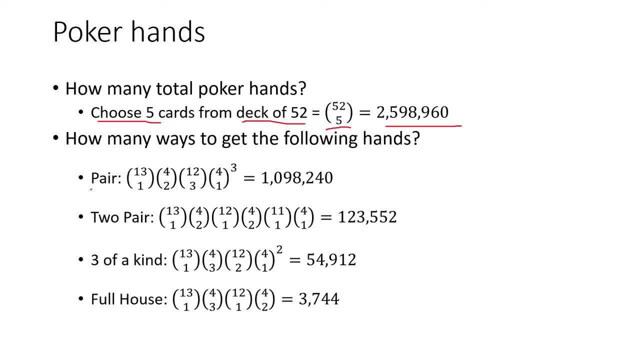 So next we can compute the number of possible ways to get a pair, for instance, and we first choose the rank of the pair. That's going to be like 2,, 3, or jack or queen, etc. There's 13 possible options there. We choose 1 and then we choose a suit for our pair, And then